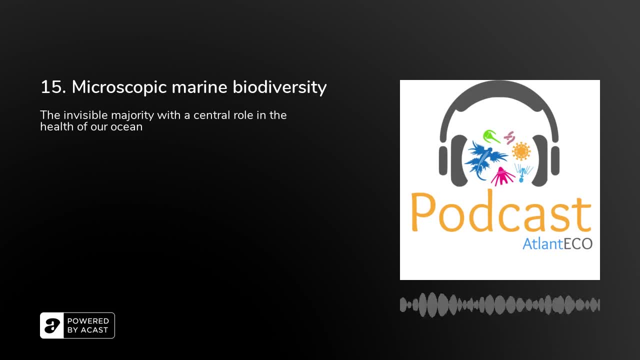 the middle of France. I went to university in the UK. I subsequently did a PhD in Belgium and I studied microbiology. I studied plants, but I only really started thinking about the ocean during the time that I was staying in the Station Zoologica in Naples, where I worked for 10 years. 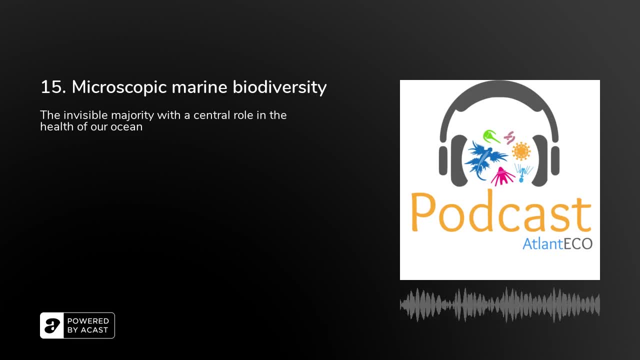 in the 1990s And being a marine biological station of quite some international renown, this is where I sort of started getting curious about the ocean and thinking about, you know, what me as a scientist could contribute to understanding more about ocean life, And as my particular interest is photosynthesis and 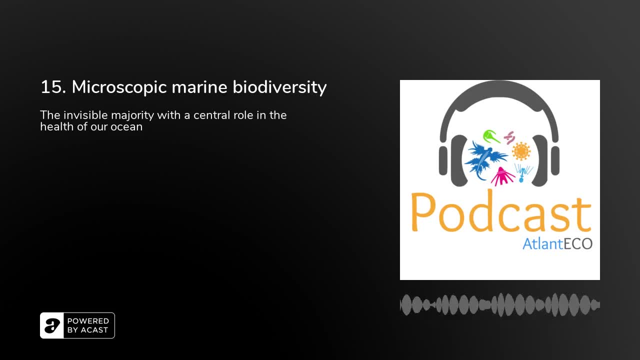 photosynthetic organisms, I started studying the phytoplankton in the ocean, which are the plants of the ocean, basically. So there you go. It's a bit of a contorted journey, as it often is in science, but a very enjoyable journey nonetheless. 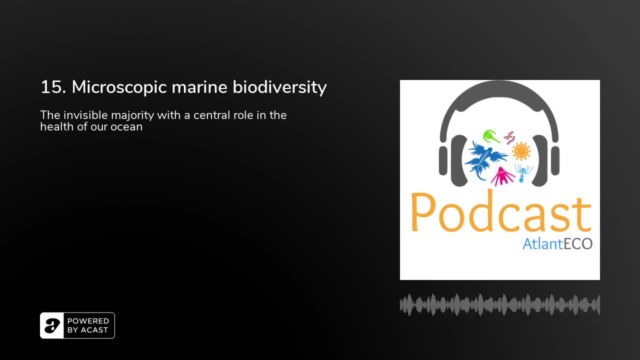 Excellent Thanks for sharing that. And in today's episode we want to talk about biodiversity And we should probably start off from a wide perspective before zooming in towards the specific kind of biodiversity that we study in Atlantico. So maybe to start with, could you? 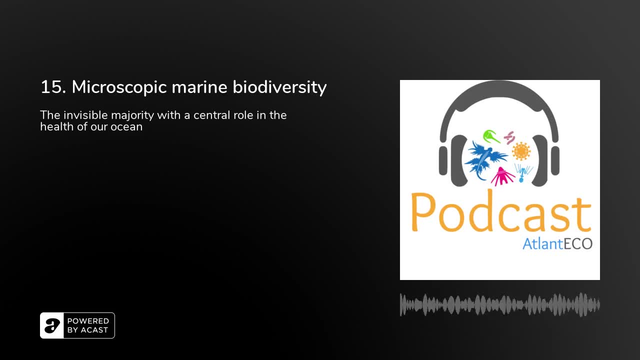 explain what marine biodiversity is and what role it plays, not only in the ocean, but also for us on land, Right? Well, first of all, let me ask a question: What do we think about when we think about marine biodiversity? I think most people 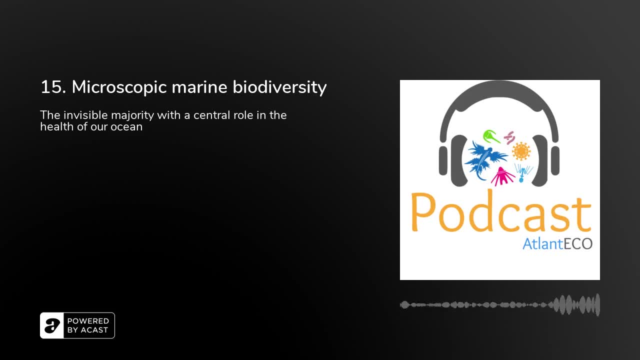 would typically think about, you know, coral reefs. They'd maybe think about dolphins and whales and the sorts of things that we typically see on TV, that we associate with marine biodiversity. And, yes, all of that is important, But in fact, the majority of biodiversity, the majority of life, 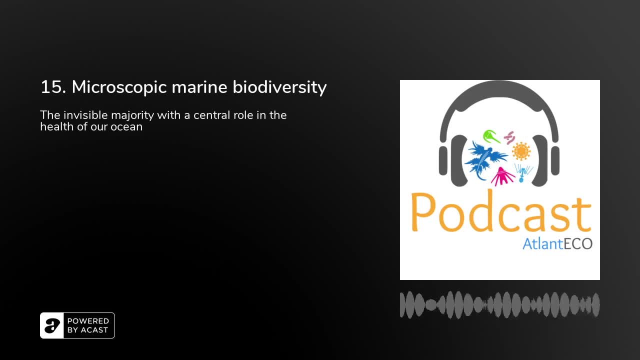 in the ocean is microscopic. This is not what you see on TV typically, But in fact two thirds of the biomass, the weight of carbon in life in the ocean, two thirds of the biomass is microscopic And that is our interest in particular in the Atlantico project And there. 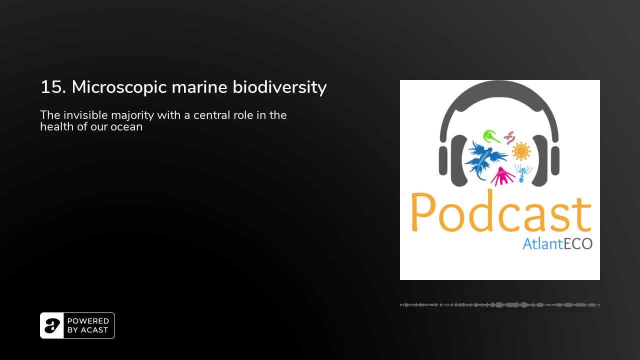 are all kinds of organisms that make up this microscopic world. It's particularly important to understand these organisms because they essentially determine the well-being of the ocean, And so this is what we want to learn more about when we're studying these organisms: How, what sort of functions do they do in the ocean? How do they determine the well-being? 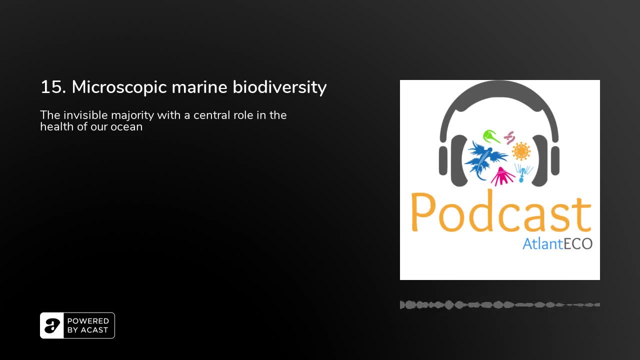 of the ocean And what happens when the marine microbiome doesn't work well. So, in a nutshell, that is our, that is our sort of interest. Now, when we think about biodiversity, we can think of biodiversity in terms of different metrics, One way of thinking of. 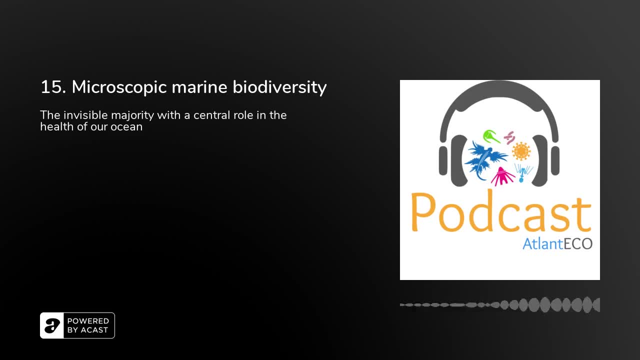 biodiversity is simply number of species on land. which is the most dominant group of organisms In terms of number of species? think about it for a second. The answer is insects. All right, Insects is a group with by far the highest biodiversity on land. Okay, What is the group? 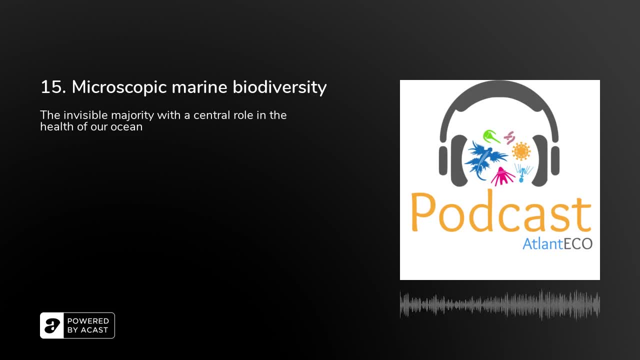 of organisms that are most biodiverse in the ocean. They're actually called diplonemids. They're microscopic. You've never heard of them. We never heard of them before making this discovery. We think they're sort of parasitic. We don't really know. So the 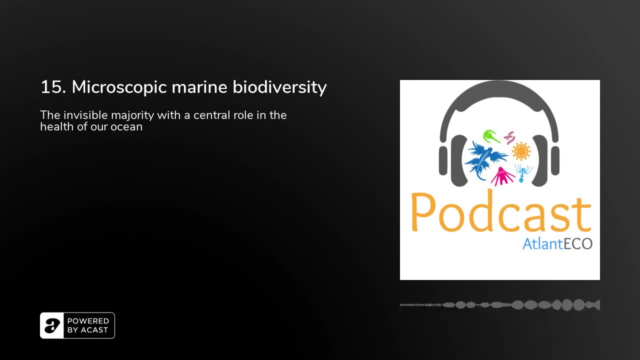 diplonemids are the insects of the ocean, microscopic organisms, which is quite pretty much unknown and unappreciated, I think, to pretty much everybody. Another metric of biodiversity is abundance. abundance of organisms, the actual weight of organisms. So which are the most? 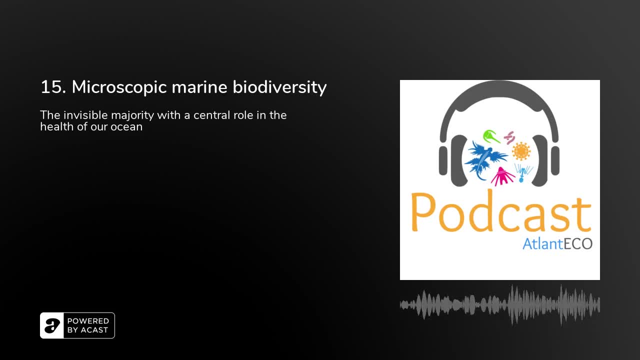 abundant organisms on land. Think about that for a second. The most abundant organisms on land are not insects, but they're not insects. They're not insects. They're not insects, They're not plants. Okay, On land the land is green. So the majority of biomass, of biodiversity on land, 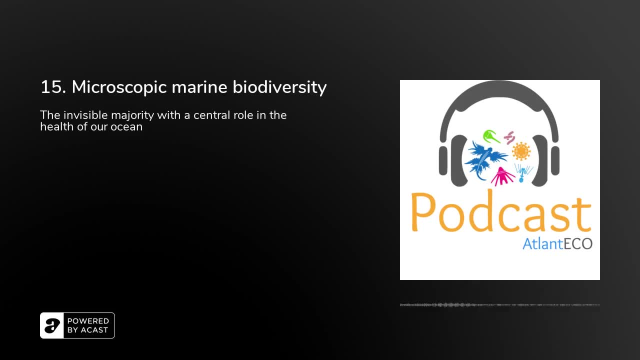 are the plants. So a very different metric to the insects In the ocean. what are the most abundant in terms of biomass in the ocean? It's not whales, It's not corals, It's not what you might think it is, but it's actually a group of organisms called radiolarians. These are again. 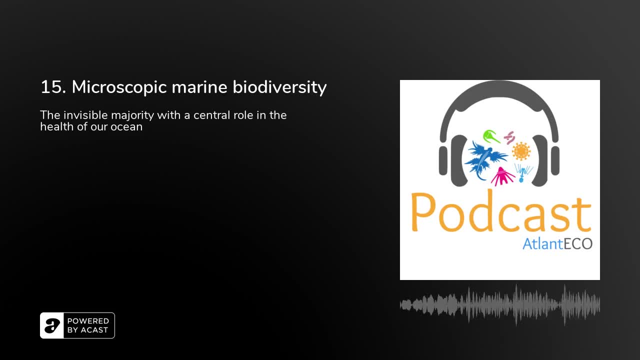 microscopic organisms underappreciated, but these have the most amount of biomass in the ocean: the radiolarians. So there you go: differences in terms of land and ocean and biodiversity in general, Wow. So that's a lot to take in and kind of makes us wonder. 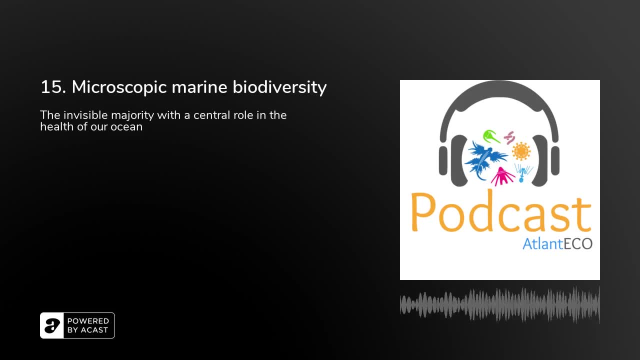 you know what we know and what we think when we think about the life on earth and life in the ocean. You know, as you said, we don't hear about these organisms and they make up a lot of our world, Exactly, Exactly. So if we get a closer look into the ocean and towards this specific 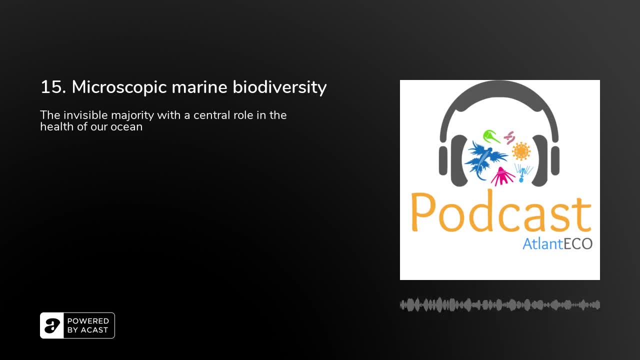 part of life present in the ocean: the microbiomes, those microscopic organisms that you were mentioning. when we talk about marine microbiome, what exactly are we talking about? Which organisms are we talking about, Right, OK, So when you look at the ocean, you don't necessarily see it. 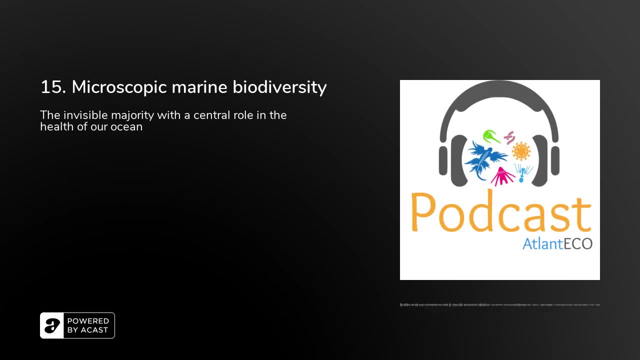 teeming with life. right When you, when you go into a forest, you see the plants, you see the animals, you see the insects. But in the ocean it looks kind of empty. And that is because actually the biomass of life in the ocean is something like 100 times less than it is on land. But 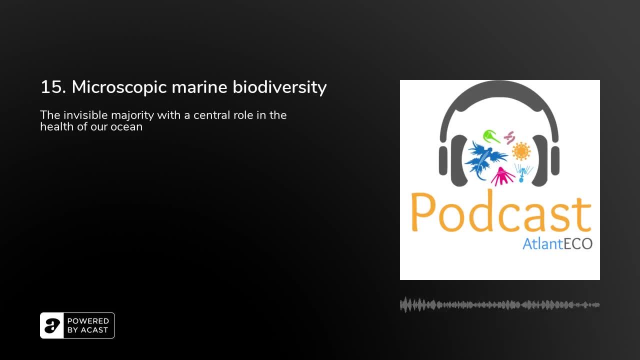 nonetheless, it's full of lots of organisms that have equivalent functions, as we find on land of equivalent importance. So, for example, one group of organisms that we have in the ocean are the photosynthetic organisms, the plants. Now, you don't really see the plants in the ocean. besides, 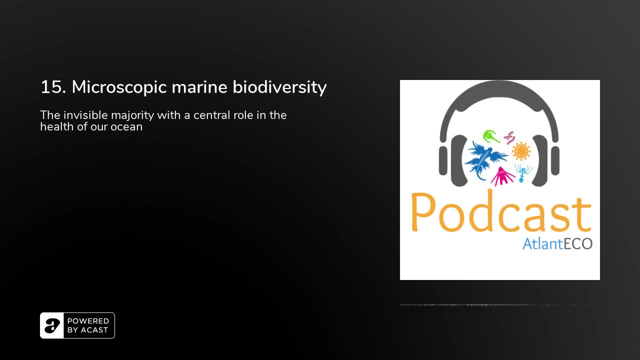 the seaweeds, the macroalgae when you're by the coast. But the majority of plants of photosynthetic organisms in the ocean are microscopic. They're single cells. But even though they're tiny, we need a microscope to see them. They're actually. 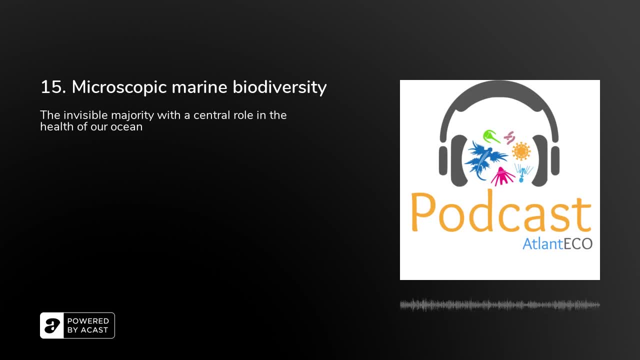 responsible for 50 percent of the photosynthesis on our planet, So they have an equivalent importance as all of the forests and fields on land in terms of the amount of photosynthesis being performed. Photosynthesis means organic material that is generated which provides food for the food. 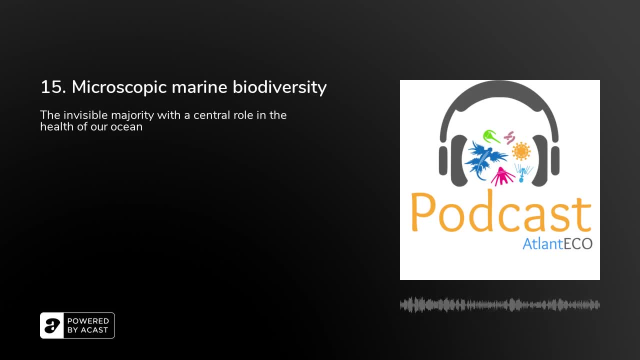 photosynthesis also means oxygen, which is generated by photosynthesis which a lot of organisms breed. And so, in all these different ways, the photosynthesis in the ocean performed by these tiny microscopic phytoplankton is exactly the same as the photosynthesis of all of the trees. 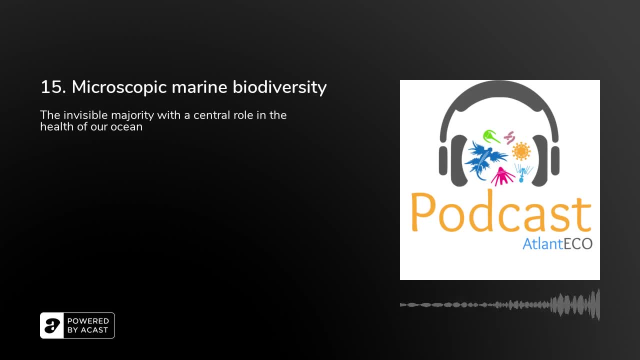 and the plants on land. So we have this group of photosynthetic organisms. They're very diverse, very interesting to study. That's what I study. in particular To these photosynthetic organisms, we have organisms called zooplankton. So zooplankton. 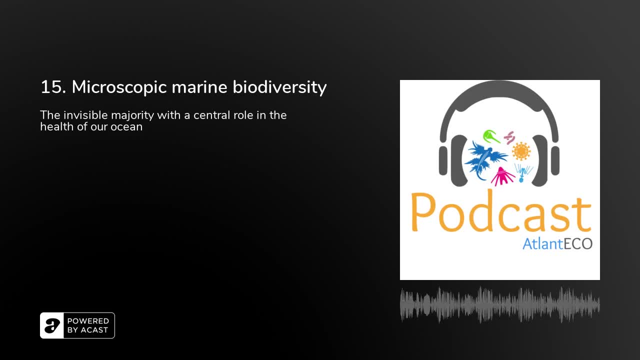 can be like herbivores. These are sort of the equivalent of the cows and the sheep, but these are also microscopic. They eat the microscopic phytoplankton and they can be single-celled. They can have multicellular structures like copepods, small jellyfish. 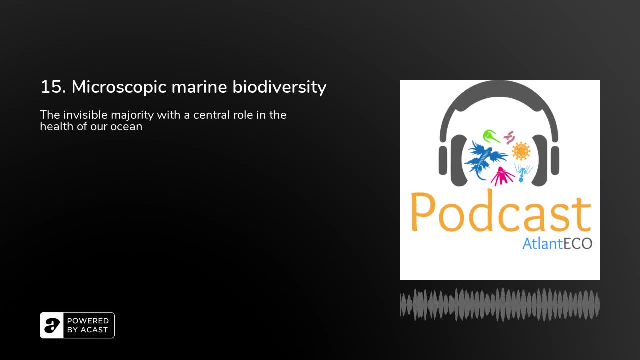 things like that: gelatinous organisms. They may be herbivores eating the microscopic plants, They may be parasites, They may be pathogens. They have all kinds of different lifestyles. In addition to these, we have also bacteria. We have lots and lots and lots of bacteria in the ocean. 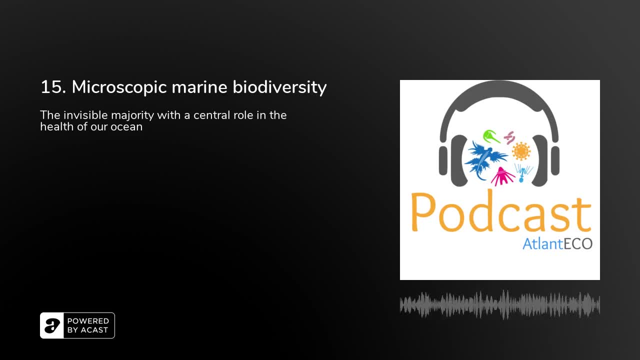 Some of these may be photosynthetic, like cyanobacteria, and some of them are not photosynthetic, but they consume sugars. They consume organic material that is present in the ocean. to recycle the organic material in the ocean. essentially, Their job is to recycle. 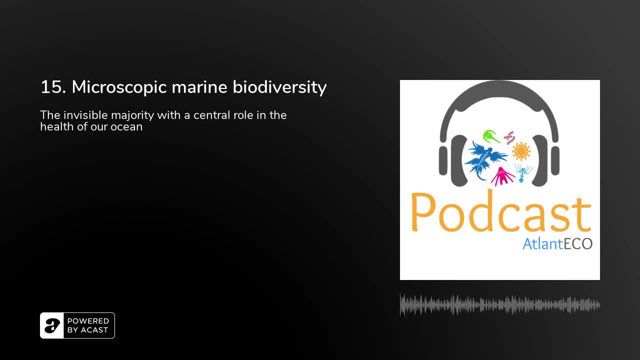 the material. In addition to the bacteria, we also have viruses. Viruses are the smallest component of living material in the ocean. But just because you're small doesn't mean you're not important, And we all know with the COVID crisis. these days we see that even the smallest organisms can be. 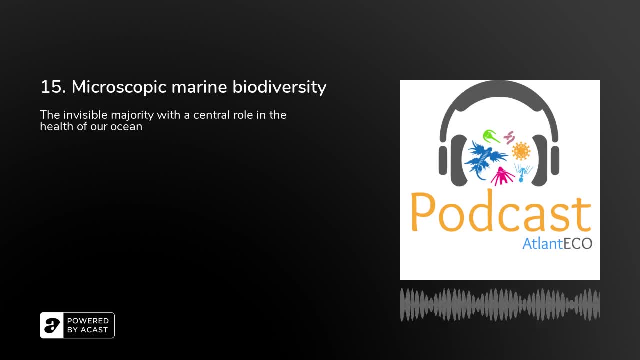 incredibly powerful, So the viruses are also very important in this microscopic world. When we consider the marine microbiome, we tend to think about all of these organisms and try to understand how they work together within this microscopic ecosystem that is so important to determine the well-being of the ocean in general. This is also kind of equivalent to the 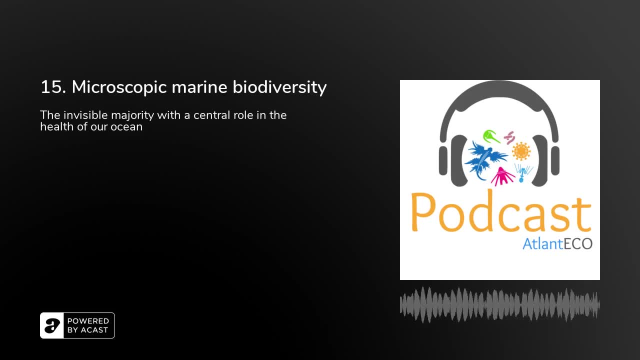 human microbiome, which may be many people more familiar with. The human microbiome consists of microbes that live in our intestines, that live on our skin. There are trillions of cells of bacteria on and within us And they really determine our state of health And they also determine our sort of 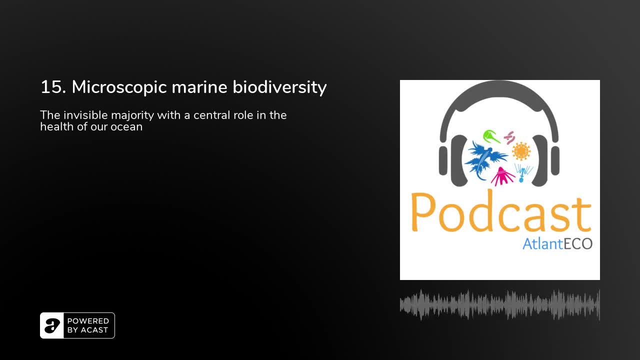 state of well-being. There's even studies showing that you know what the microbiome is doing on our skin or inside our guts determines, sort of you know whether we wake up feeling good or whether we wake up feeling lousy and so on. So microbes, even though they're small, they're incredibly. 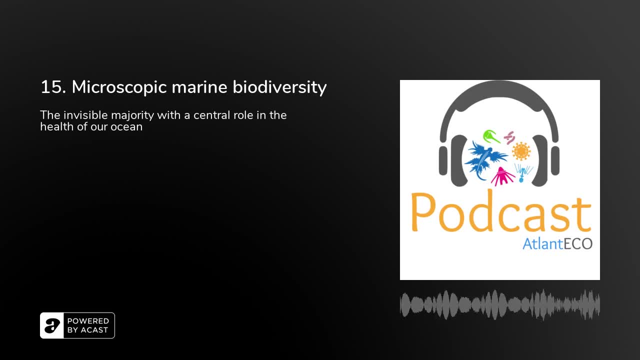 important for everything, really, The functioning of all of us, And so, you know, we've got to think about all of the life on our planet, and including ourselves, of course. So they are, as we've seen in a previous episode that was introducing, you know, the marine microbiome. 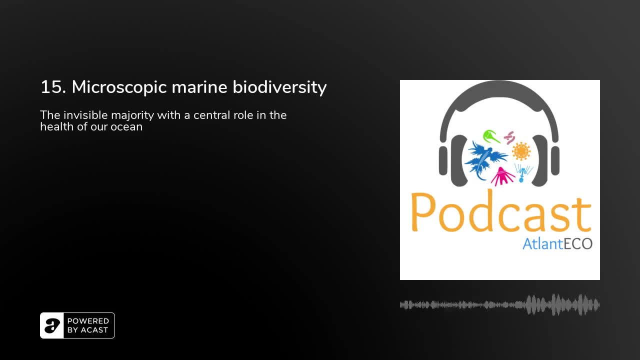 they are the start of the food chain. Yeah, as you say, really important in the cycle of life. Yeah, they are the start of the food chain, channeling organic material up the food chain to the larger organisms. And they are also the recyclers: They decompose material in the ocean. 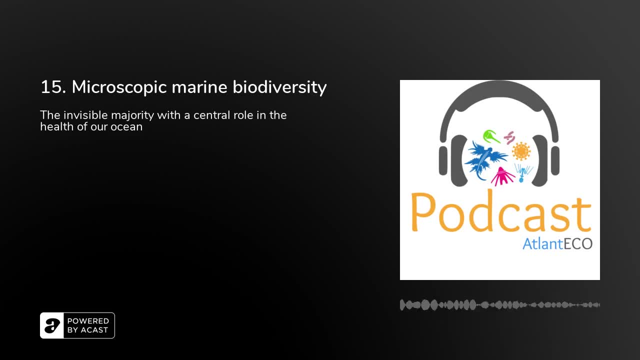 They recycle material. So these multiple functions are really important, as we know, in sort of the functioning of our own daily lives. Yes, we need to eat, but we also produce garbage which needs to be recycled to ensure that the whole system can function in sort of a circular way And the microbes in the 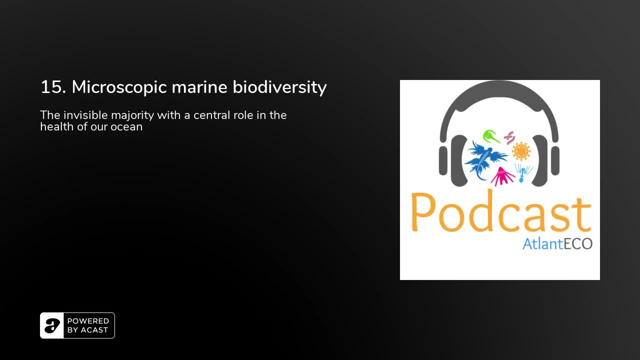 ocean do that, assuring the functions in different ways of the whole system such that it can be healthy. Yeah, yeah, And so you know, we've got to think about all of these things And I think that's a really important. 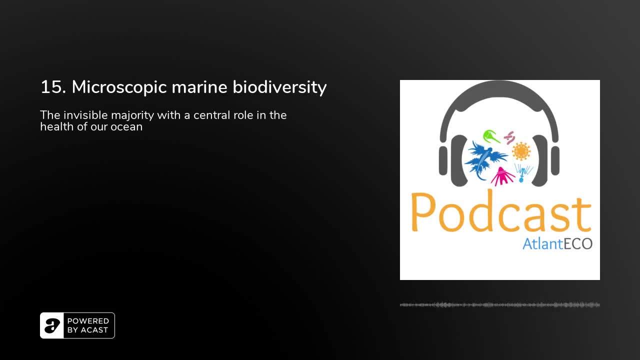 thing, Yeah. So to come back, maybe to Atlantico, in the project we study these organisms with genetic and genomics techniques. So first of all, can you explain what these techniques are, What does it mean, And secondly, what do we already and what will we learn from applying these to the? 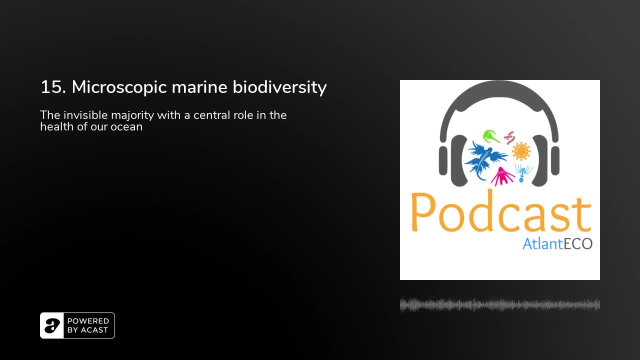 marine microbiomes that we find in the Atlantic. Yeah, so because these organisms are microscopic, we can't see them with the naked eye Like we can see life in a forest. when we go to study a forest ecosystem, We need special tools to visualize these organisms, One set of tools that are incredibly powerful are based on what? 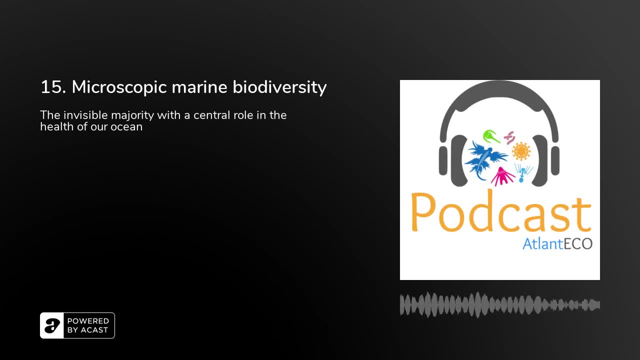 we call genomics, which is basically DNA-based studies, So sequencing of DNA. All organisms contain DNA or nucleic acids. It consists of just four letters, Okay. so, unlike our alphabet, which has A, B, C, D, E, 26.. 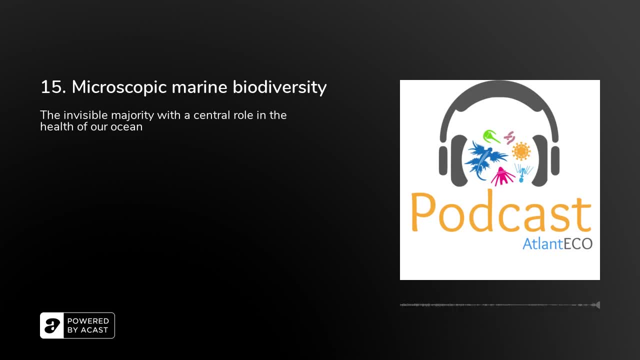 The alphabet of the genome is just four letters: G, A, T and C. All organisms possess those four letters and they possess very long strings of those letters. And by studying those strings of Gs As Ts and Cs we can divine sort of what we call barcodes of organisms. So just like you go. 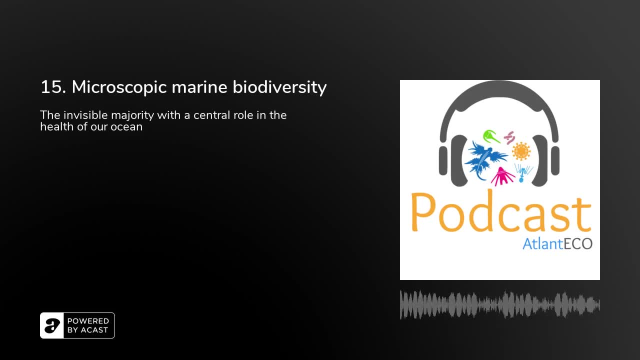 in a supermarket, and a barcode can be used to indicate where a product comes from, how much does it cost, et cetera. The barcodes of DNA are very useful to tell us the identity of a species and to tell us what sort of functions it may perform, So the DNA is incredibly important to provide us with these. 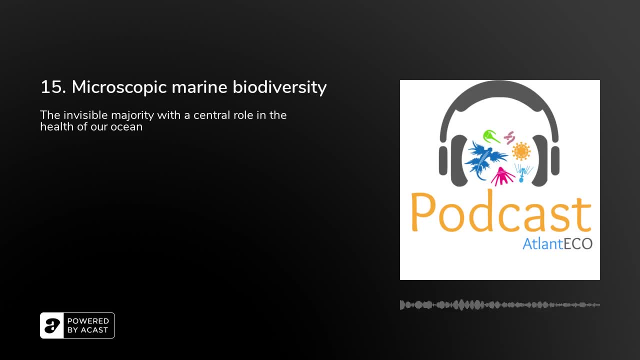 barcodes that allow us to identify all of these different organisms that are present in this microscopic world. And there are millions of different organisms, So it's a very complex process to dissect, disentangle all of that DNA-based information. But fortunately these days we have a lot of young people that are very smart in computer. 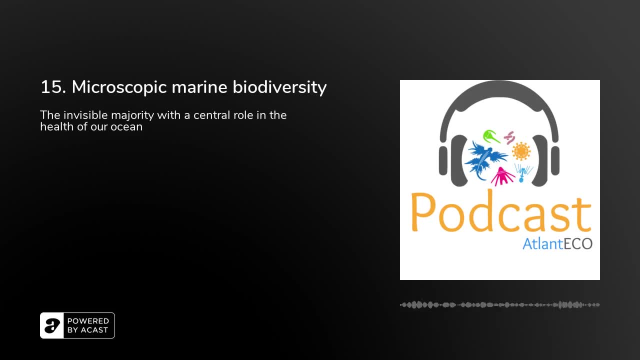 sciences and they do the job to disentangle all of this huge array of DNA-based information, which is great. But, at the end of the day, DNA sure is very powerful, but it's still one-dimensional at the end, right, It's just a string of Gs As Ts and Cs, So it's not sort. 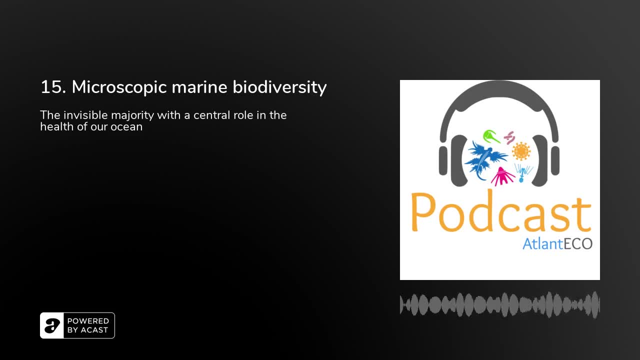 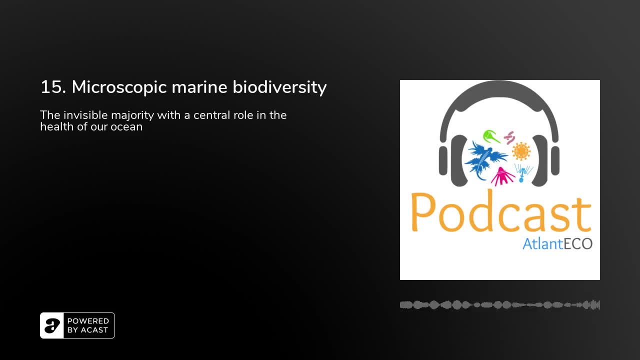 What organisms are present in this microscopic world and what are they doing? And one technique that we use a lot in Atlantico is microscopy. So microscopes just like telescopes. they allow us to see things that the human eye cannot see. Microscopes have been around since the 1600s. 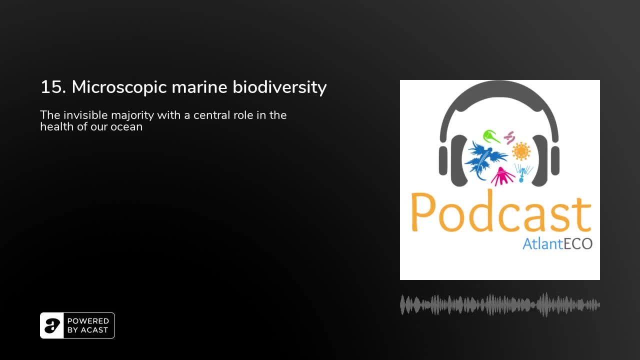 but these days the microscopes that we use are incredibly powerful. They allow us to see sort of the outside of cells and they allow us to dig deep into the interior of cells to see all kinds of different things. So by adding together the one-dimensional DNA-based 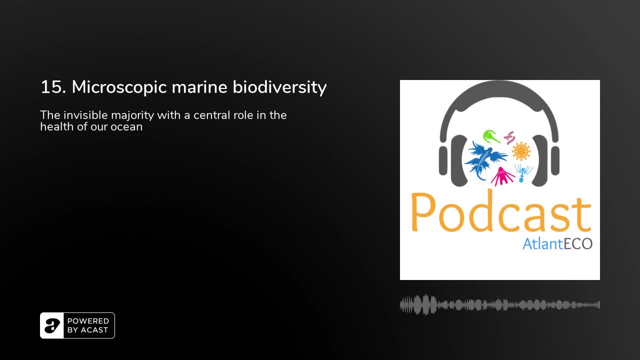 information. with the three-dimensional microscopic information we can get a pretty complete picture of all of the organisms that are present in different marine environments. So that's sort of what tools that we use to explore these invisible ecosystems. Nice, And what can we hope? 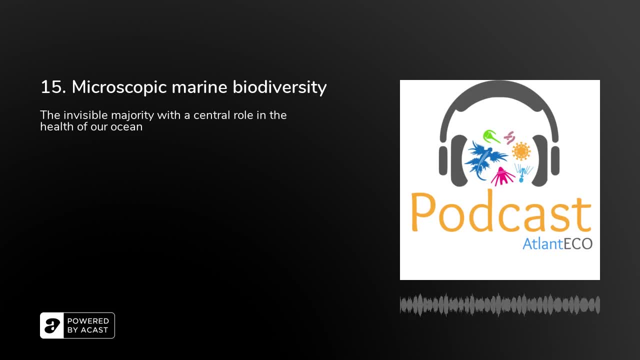 to learn from Studying these animals in all those different dimensions. Yeah, a couple of examples, what we can use this information for. One example is: these organisms are an incredible bio-resource of new genes, of new molecules. You can think of this as really. 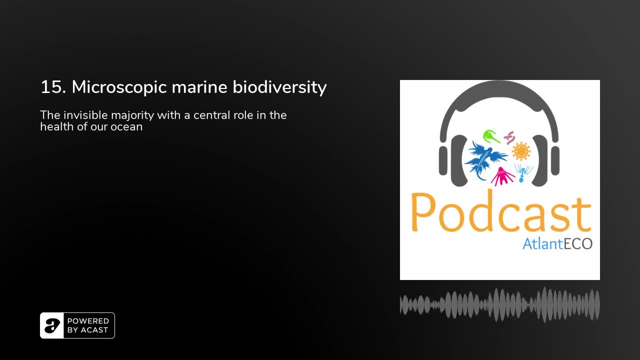 the treasure trove of the ocean, These microscopic organisms. they have thousands of genes, many of which we don't know about yet, that encode for different processes in the cell. And some of these processes we can think to use and exploit in our own daily lives, For example. 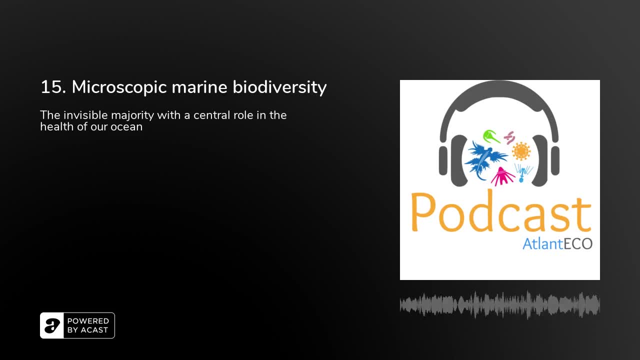 to develop new drugs for beating cancer, for beating diabetes, against some of our terrible illnesses like Parkinson's, Alzheimer's. We can try to look for these drugs in the ocean. We can also find new materials that are useful in our daily life, like adhesives, like glues, like abrasives. 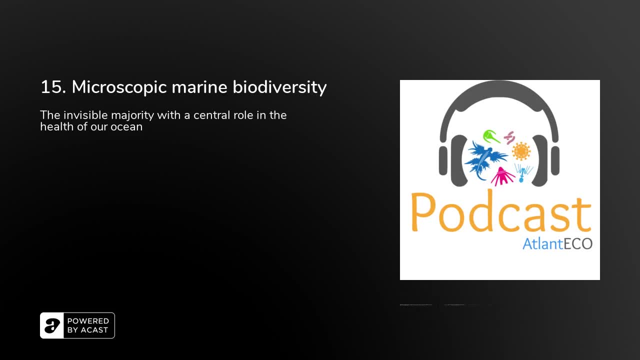 all these kinds of industrial materials which today we derive from petroleum, from fossil fuels. We could hope to replace the fossil fuels with these kinds of natural products in the coming decades. we would hope So. that's one sort of resource that we can imagine from this treasure trove of organisms in the ocean. And another thing: 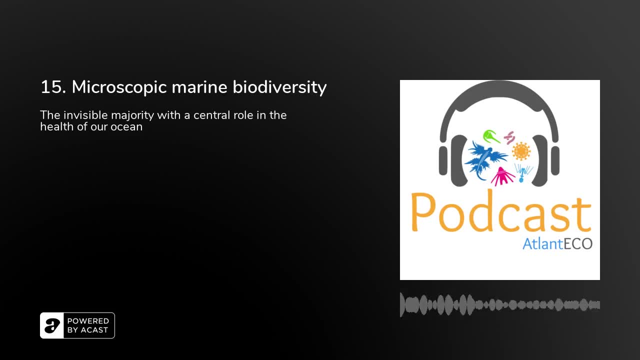 that we could try to do is to use the information from the ocean microbiome to define a sort of microbiome health index for the ocean. So, as I say that these organisms, these communities, determine the well-being of the ocean, If we could use these organisms as sort of a diagnostic, if we could, you know, categorize these communities and define, you know, a healthy ecosystem by the organisms, by the activities that are happening within that microbial community, and distinguish it from an unhealthy ecosystem, a polluted ecosystem or an ecosystem that is not healthy. 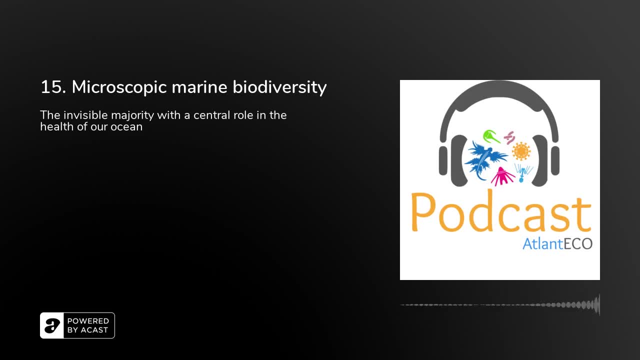 If we could do that, if we could identify the organisms that are very, very much impacted by, by agricultural runoff or by antibiotics and other chemicals coming out of cities by the coast, then we can use these organisms as what we can call a microbial health index. 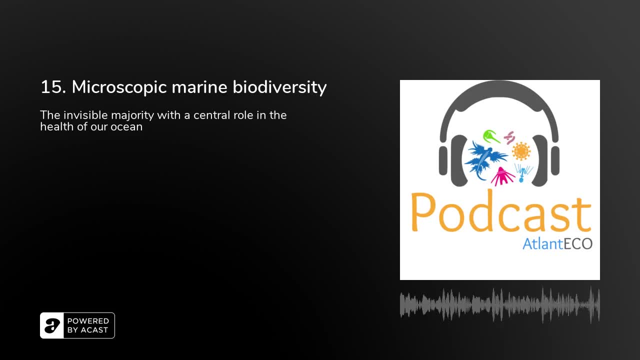 So just by doing DNA-based analyses of the microbial communities we can define a gradient of healthiness of the ocean which can help us then implement measures to measure the health of the ocean, maybe make an ecosystem more healthy by intervening in agriculture, by intervening 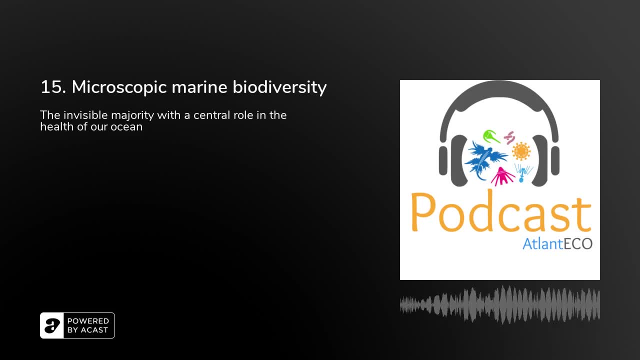 in other processes. So this is how we could sort of hope to develop sort of a diagnostic tool where we use these microbes to tell us about the health of an ecosystem And also as a preventive tool, by monitoring a microbiome health index. this would allow us to perhaps spot alarm signals. 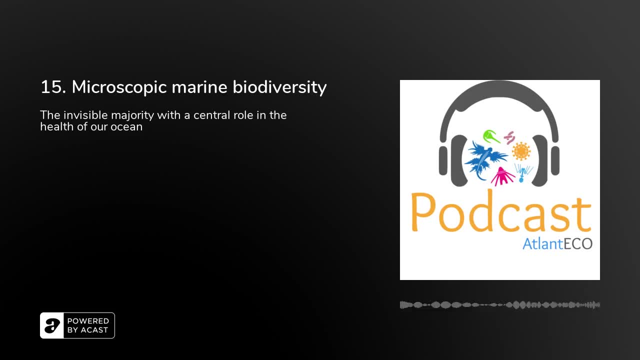 before they manifest themselves in more catastrophic ways. So the health index of the ocean, based on microbial content of the ecosystem and the activities of the microbes, that could be a very promising approach for the future. I think These things are all interesting in the context. 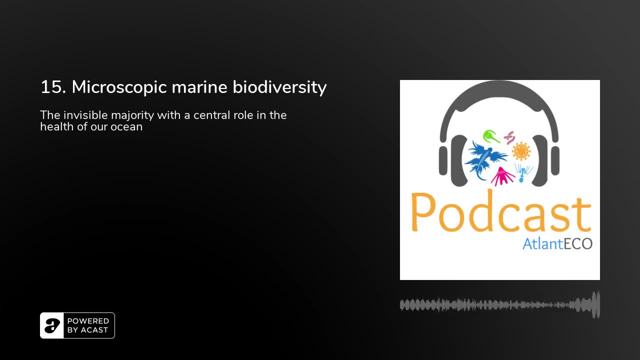 of the Atlantico project? Yeah, for sure. And because we study also the environment within which these microbes evolve. if we put all of this information together, what we hope for is to develop these models that can help us sort of predict the status of the 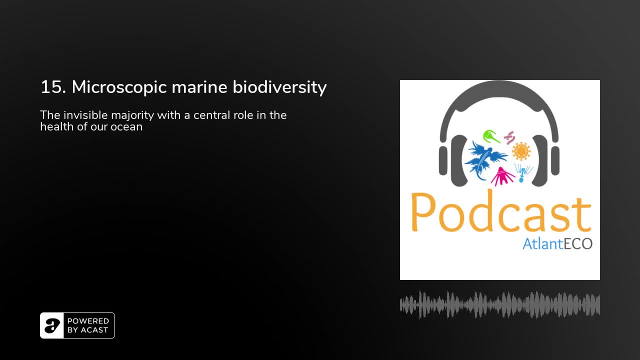 ocean in different regions of the Atlantic And, as you say, you know better, manage what is happening, prevent maybe some bad things from happening in regions before they actually happen. That's amazing what we can learn from these tiny, tiny things that we can't even see Exactly. 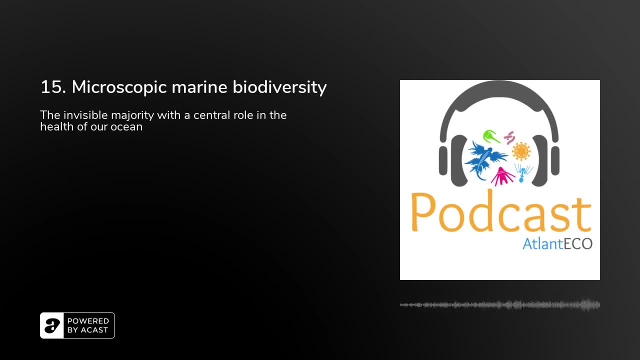 And maybe to finish with, if we want to look into the future and just asking you know, in your opinion, what could we expect in the coming years in terms of new technologies for studying the marine microbiomes? Is there anything coming up on the horizon? 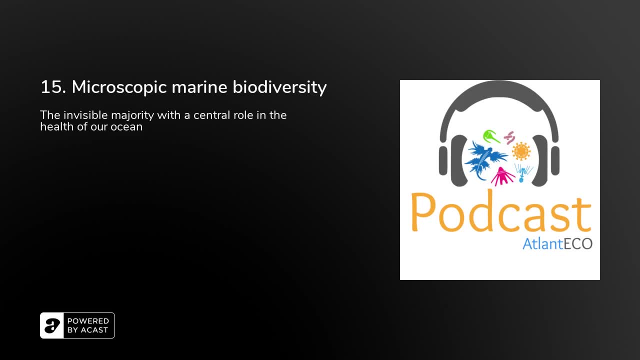 Yeah, there's lots of things being developed And, as is often the case in science, new advances are driven by new technologies. Sometimes in science you have a huge intellectual leap, But oftentimes the advances in science are driven by new technology that comes along. 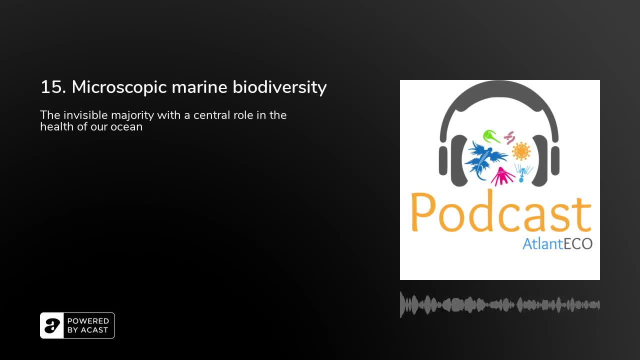 that opens up our eyes to some unexplored phenomena, In the case of exploration of the ocean microbiome. well, on the one hand, our technologies are becoming more and more powerful, Sequencing DNA, for example. new microscopic methods are getting more and more powerful. 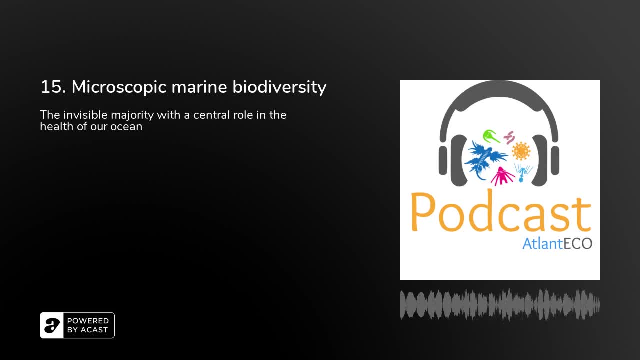 They're steadily getting cheaper as well. So for the same amount of money, you can do more analyses. This is going to continue into the future, I expect. On the other hand, some of the instrumentation is becoming smaller. it's becoming miniaturized. 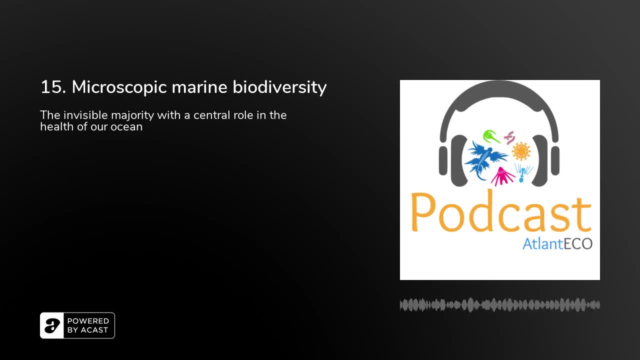 and it's becoming automated, which means that some equipment traditionally is in a laboratory on land. you can now start to think about putting it on a ship and doing your analyses rather than in a lab on land, doing them actually on board a research vessel or even a smaller vessel out at 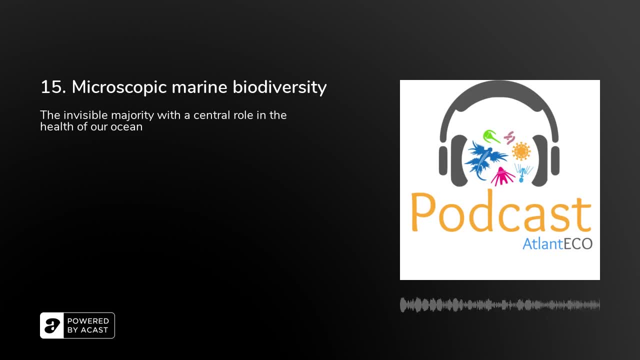 sea. This totally changes what you can do in oceanography, because you can- you know, you can- really study a phenomenon while you're out at sea. you can get the results on the same day that you are sampling, and then you can adjust your scientific questions immediately to then go. 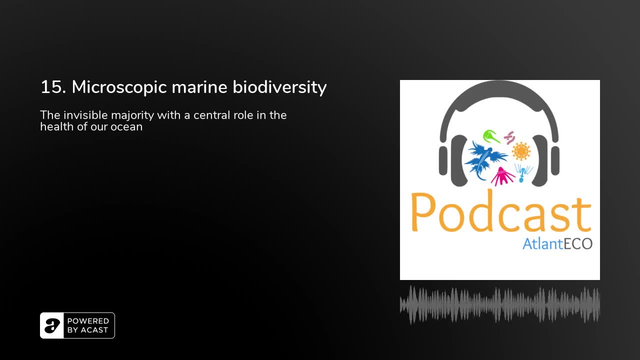 and- do you know slightly different- sampling program the following day. This completely revolutionizes oceanography, which is typically done, you know more, with back and forth between land and sea that takes several years. So these miniaturization automation are radically changing. 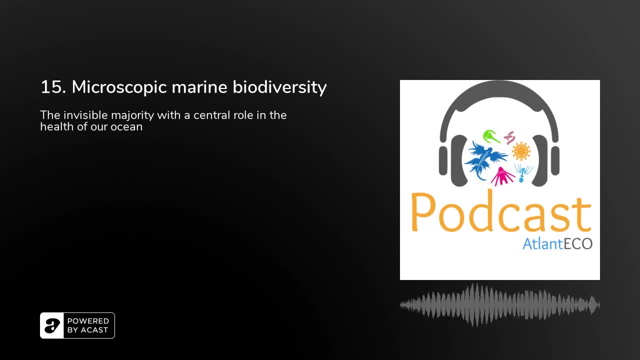 the way we do oceanography. this is likely to continue in the future And perhaps you know 10 years, 20 years. now we can actually do DNA sequencing in the water. we can image the organisms in the water on like autonomous floats that are drifting around the ocean. 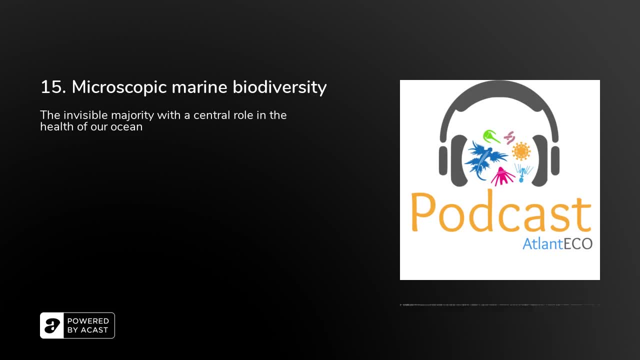 So perhaps we can study the ocean microbiome without the need for, you know, expensive research vessels going out and sampling, If we have a whole array of sensors that we put out. we can actually do that, And so you know. we can actually do that, And so you know. 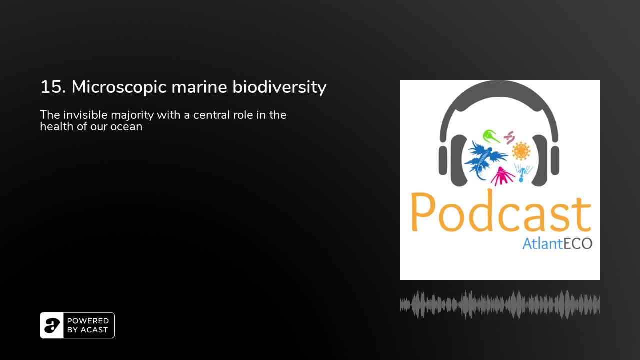 if we have a whole array of sensors that we put out in the ocean, that are steadily sequencing DNA, steadily imaging DNA actually in the water, beaming back that information via satellite back to laboratories such as myself on land, then this will again totally revolutionize the way. 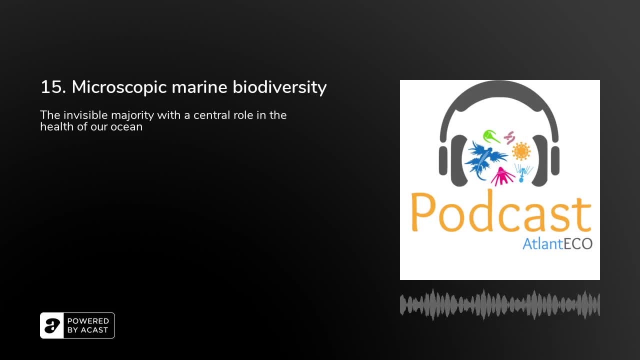 that we do science and the way that we study the microbiome in the ocean. So this will gather a lot more data than what we have today. Coming back to your point about yet the need for having a lot of data sort of at the all Atlantic level which will allow us to sort of detect warning signals of 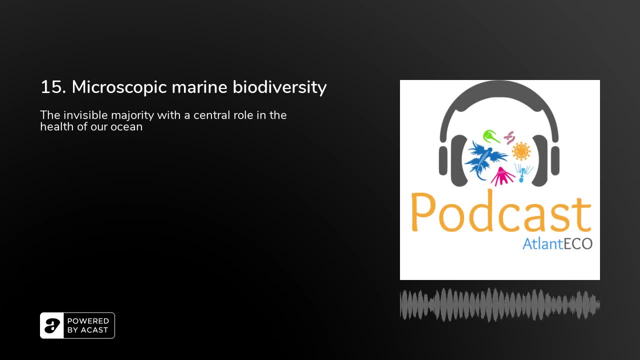 an ecosystem, in a particular environment that is starting to go haywire. By having these autonomous arrays of instrumentation deployed at sea, we will be able to gather that information, you know, ideally at sort of an all Atlantic level, which will give us then the statistical power that we need in our analyses to be able to 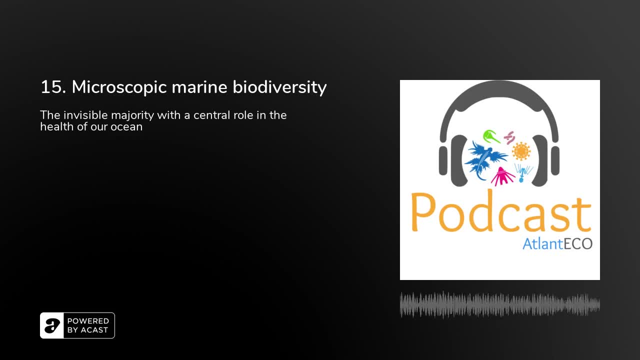 identify, yes, what really is a healthy ocean microbiome And what is an unhealthy ocean microbiome, And where are the warning signals that we can use to tell us, you know, when an ecosystem starts to get out of balance, And in what way does it get out of balance, And what could we eventually? 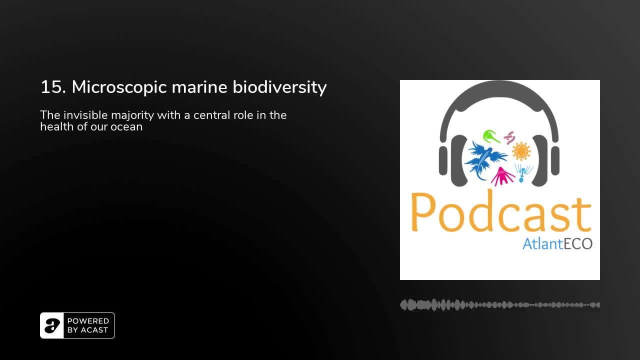 try to do to restore the balance in the future. So there's plenty of things on the horizon. certainly a very exciting time, And you don't even necessarily have to be a scientist to get involved. This miniaturization, these new technologies these days are also permitting more and more citizens to get involved in science. So 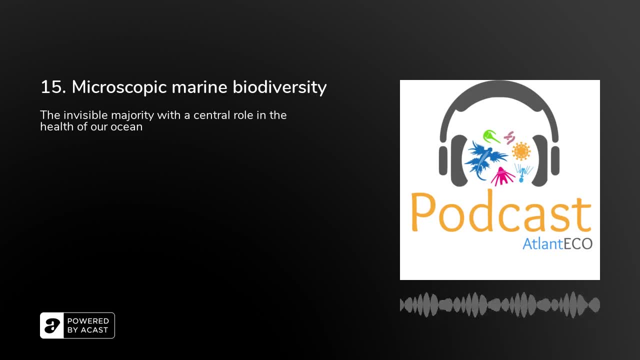 just like, you know, the general public, the interested citizens, really contribute a lot to ornithology, to looking at bird migrations in Europe, around the world, much like the general public really contributes to astronomy by identifying, you know, new stars, new phenomena. 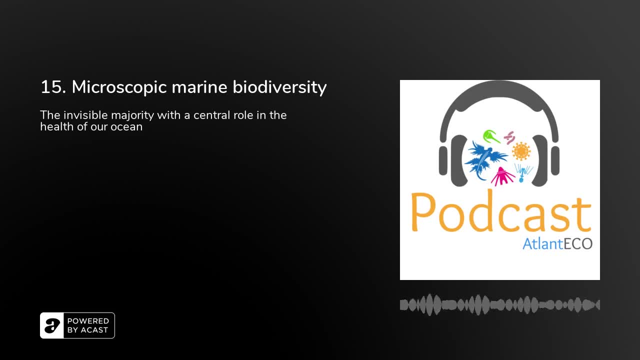 and so on. We can hope that more and more citizens will be able to get involved in ocean sciences as well: to collect samples, identify organisms using, you know, cheap little microscopes and so on. So there's plenty of ways. I think that oceanography is likely to change in the future. 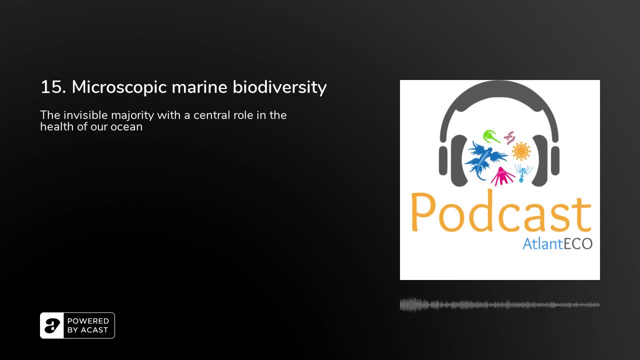 and will allow us to generate a lot more data from the ocean, which will allow us to to increase our understanding of how the ocean works and how the microbes assure the well being system. So a lot of, as you say, exciting times to be doing oceanography, and not only for the 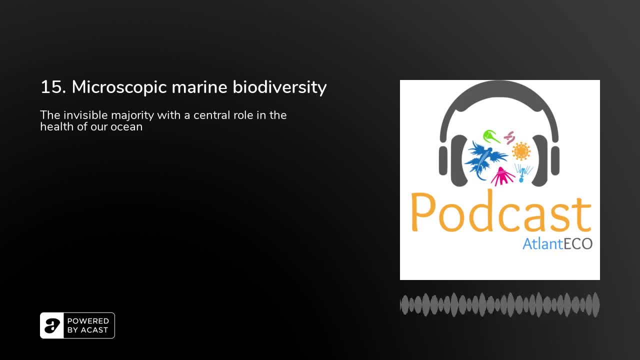 scientists, but for anyone really who maybe get their hands on the, on one of those small microscopes. I mean, those things can be adapted to your mobile phone. Now you can take pictures of of these microorganisms using your cell phone. So, yeah, indeed, And yeah, you know, as we know. 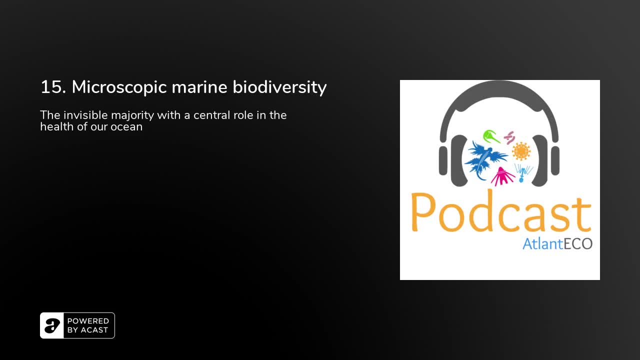 you know, seeing is believing. you know, when you look at the ocean you maybe don't appreciate all of these microbes that are present, but if you could see them, then suddenly your eyes are open to this amazing microscopic world that is so important for. 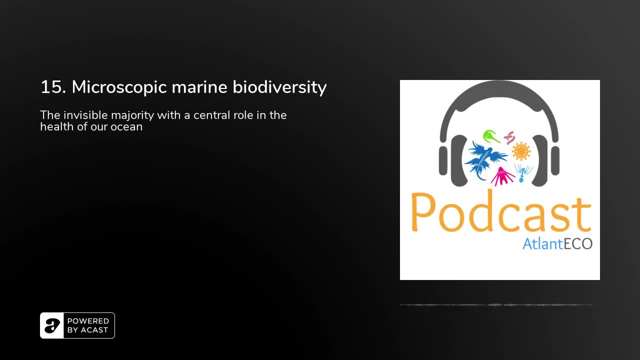 managing the well being of the ocean. And since, yeah, the ocean is our joint responsibility, we all have to play a role in looking after the ocean, preserving its well being. These new approaches will hopefully give more people the opportunity to actually participate and contribute to making the ocean the healthy, well looked after place that we all dream about. 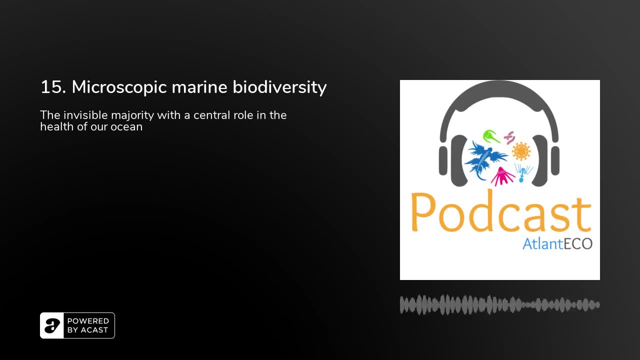 I think that's a beautiful place to end our conversation today, Chris. So I have to thank you for taking your time to explain to us what biodiversity is, which we started with, and then on our journey to understanding more about this microscopic world in the ocean and how everybody can get involved. For our listeners, we will be having some 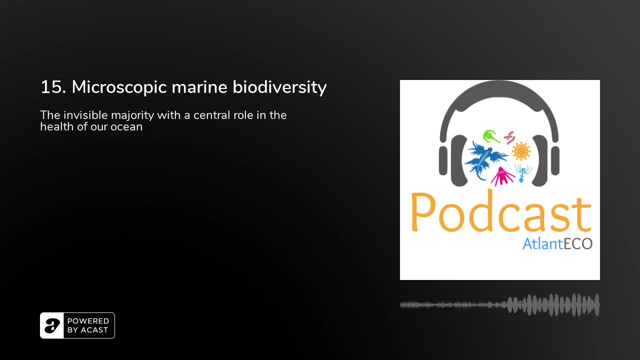 conversations with projects that are developing those sensors that Chris was talking about, and also with people that work on making those microscopes that can be used and accessed by the citizens so that they can participate in generating that data and that knowledge. So keep coming back to the podcast to learn more about how we study the ocean and how